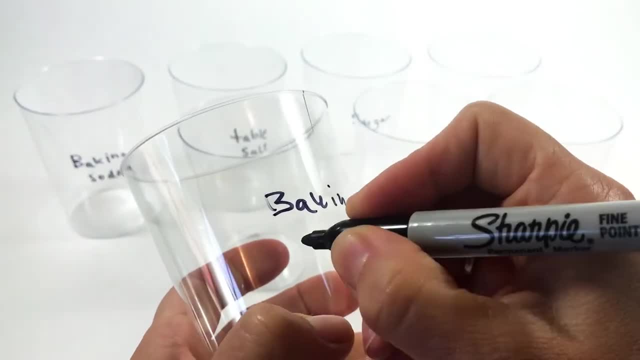 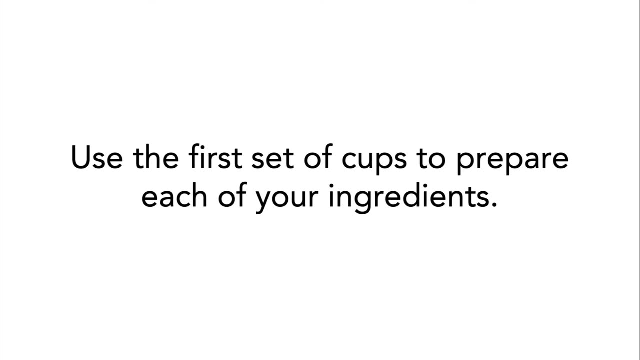 First I will introduce my camera. This camera is a camera that is used in the film. It is not made for filming. This is a bit of a surprise. This is a camera used in the film. This camera is a camera that is used in the film. 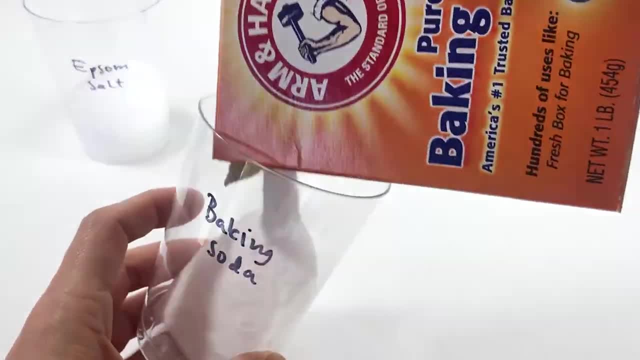 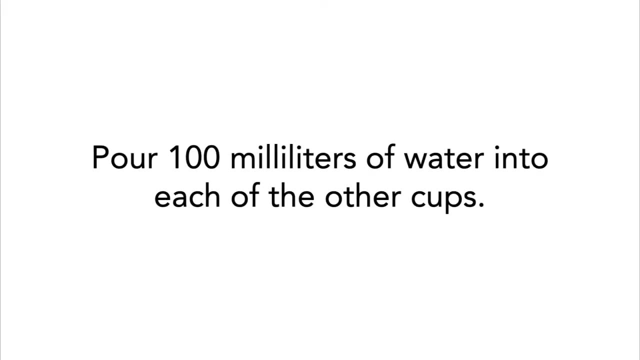 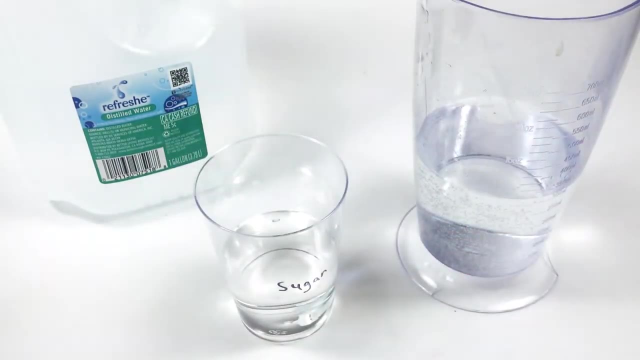 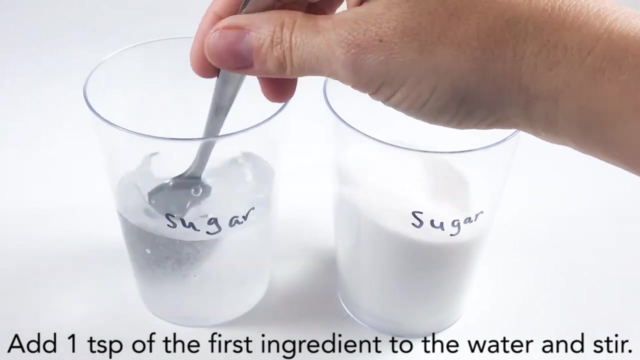 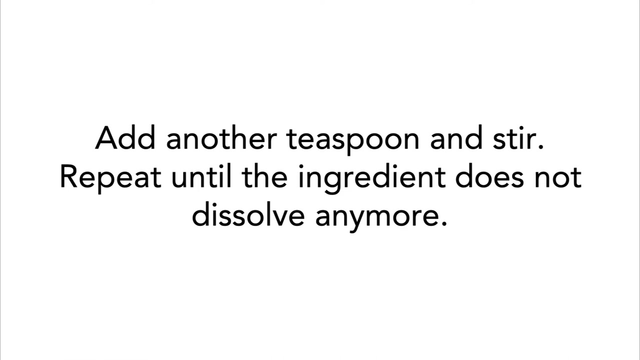 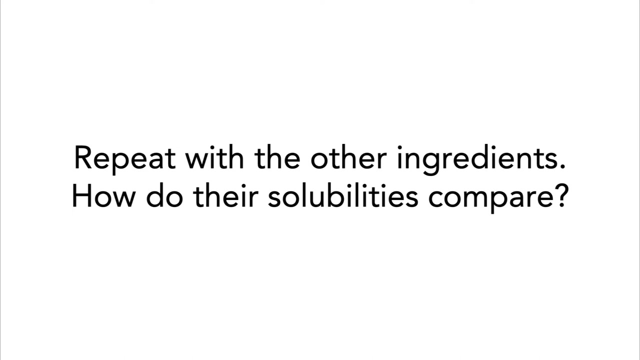 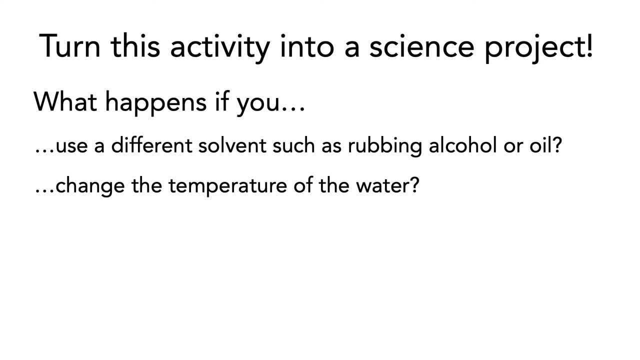 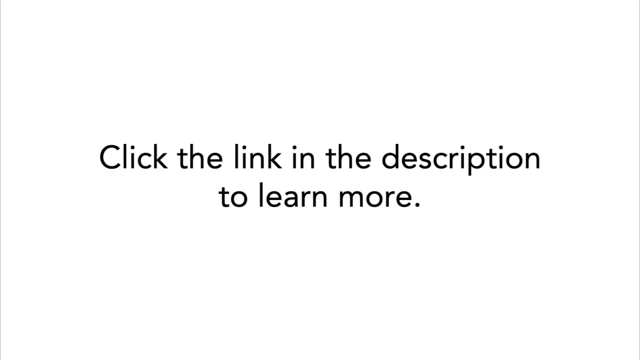 This is a camera that is used in the film. This camera is used in the film. Thank you, Thank you, Thank you. 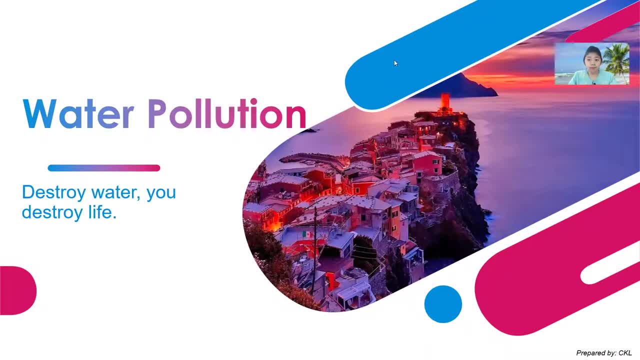 Okay, Hello everybody. So I just I hope all of you are doing well And for the last three chapters regarding the Arctic ecologies, I hope you have a clear understanding, Okay, So from your comments, I found that mostly all of you understand what I'm going to explain. 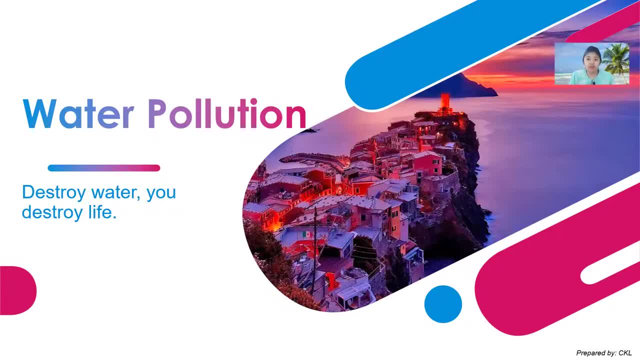 And also I want you to understand. So later I will share with you the summary for these three chapters, because I found that there is one student successful to summary the main point for chapter one, chapter two and chapter three. Right, Okay, So today's we will enter after you. 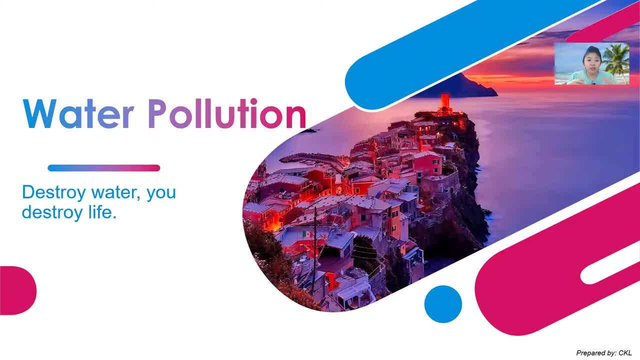